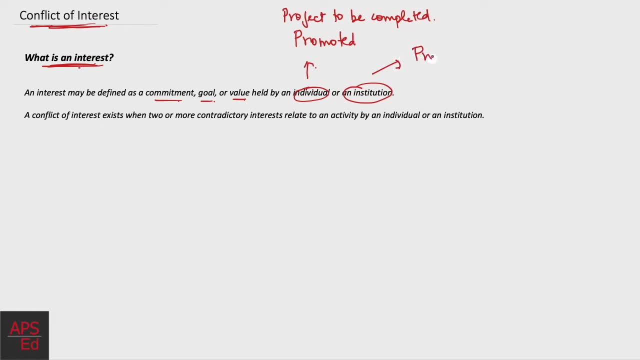 Or you want some particular project to be completed. So this all I am talking about what happens in a company, not like your general interest, an organization. the interest could be like protecting the environment. so these are some random examples which i am giving for an interest. so what is this conflict of interest as the name? 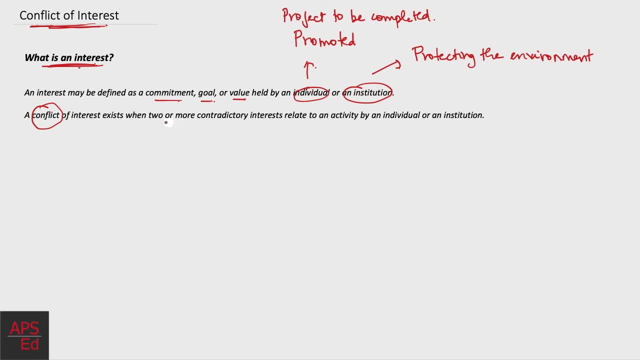 suggests there is a conflict. so it happens when there are two or more contradictory interest, like there will be two or more interest relating to an activity by the individual or an institution if those two interest come in contradiction, which each with each other, that is known as conflict of interest. like, let us say: you are having some stocks, you are owning some stocks. 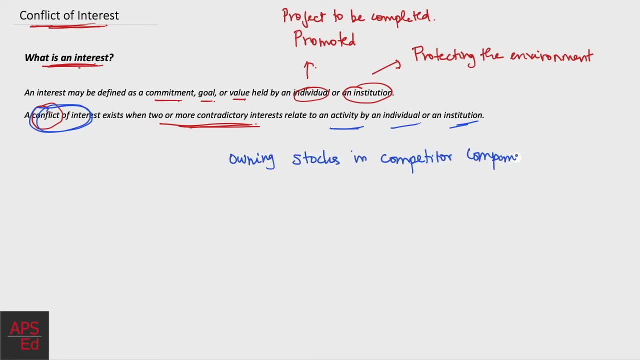 in competitor company. so let us say you are working for company a and you are owning stocks in competitor company b. so you know whatever is happening in company a and that might affect the stocks of company b. so this is obviously a conflict of interest like you are having. you are working for a and having 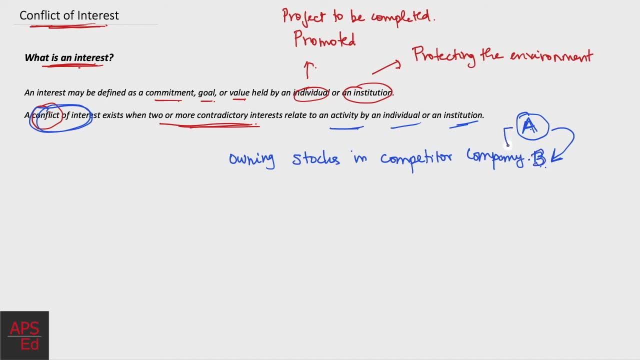 some stocks in b also which are against each other. like any activity in a will affect b and any activity in b will affect a. so this is one conflict of interest. another is inside information. so recently you would have heard that this jet airways went down. the stocks went down. 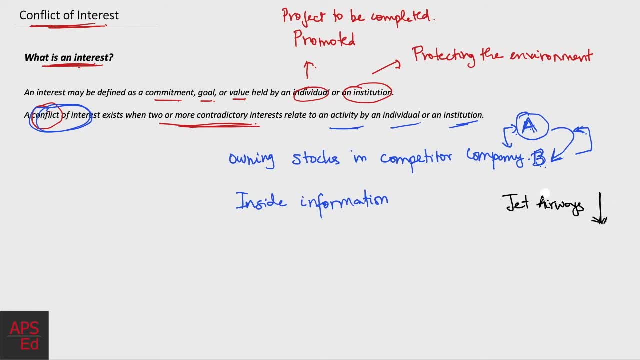 and and even the airline shut down. as an employee of the company, you know that this is bound to happen, that jet airways is bound to shut down, like you know this inside information, but what you do is you pass it on to others. let us say: you are the employee of, you are an employee of jet airways. 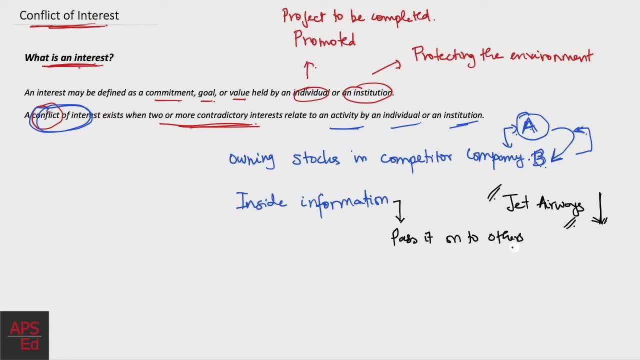 and you know that it is going to close down and you pass that information to me. so what? what i do is, whatever stocks i own, i sell it off or spread this information. so this inside information creates a conflict of interest. like you are not being loyal to the company and whatever secret.